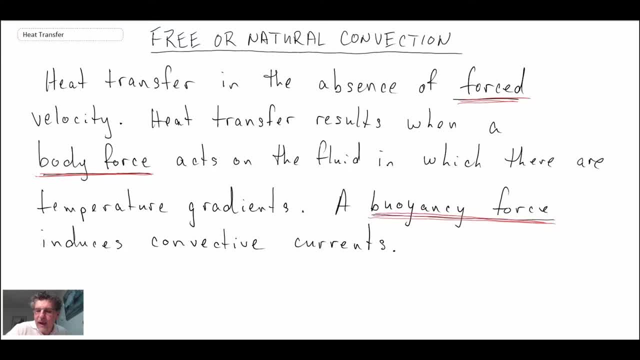 being hot, in which case, typically, with the gas or liquid, it will be less dense and it will move up, Or, if it is cooler, it will become more dense and then it will drop or descend, And that becomes the mechanism by which we can have what we call convective current. So what we're going to do, 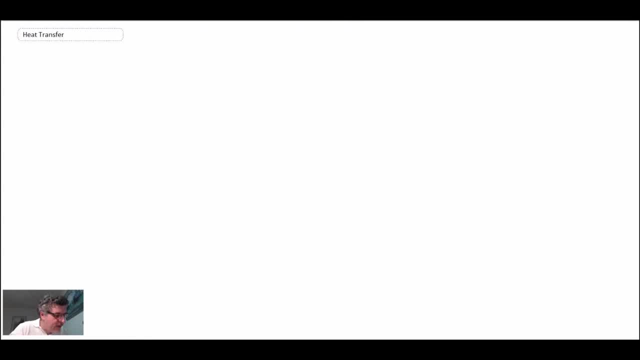 we're going to begin by looking at some common engineering examples where you could have free or natural convection. So the first one that we'll look at, or electronic cooling packages or fins, And then we will look at another form, which is natural convection on the back of 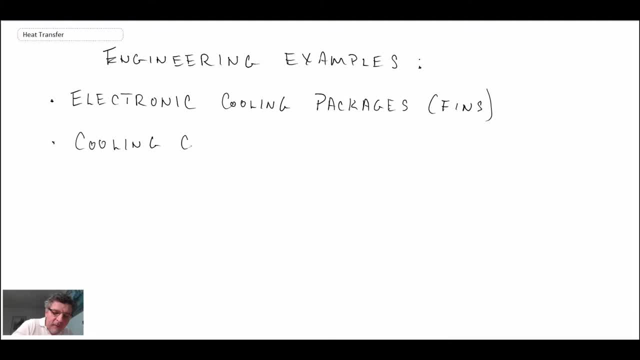 refrigeration systems or refrigerators. And the last thing that we will take a look at is heating systems, And these could either be electric, where you have dual heating, It be where you have hot water circulating, or you could have steam. so let's go ahead and start. 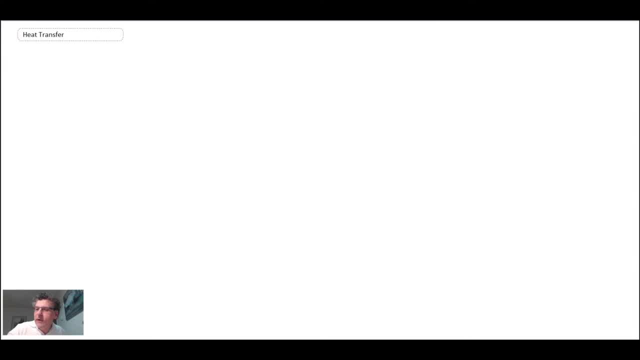 looking at some of these different applications where we would have free or natural convection, and what we'll begin with. we'll begin with electronic cooling, and so here we can see the fan on the motherboard of a computer and that's a pretty standard thing that has connected heat. 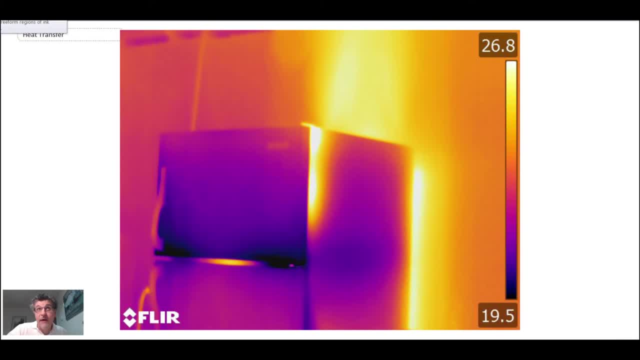 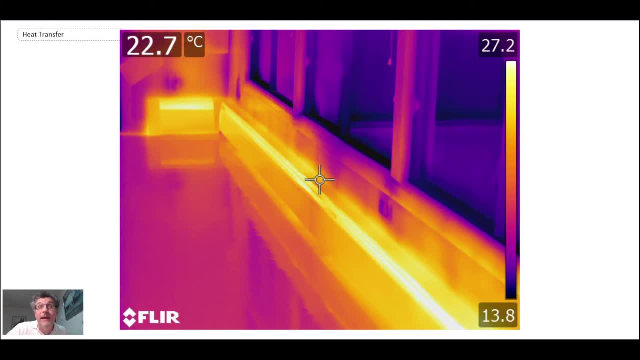 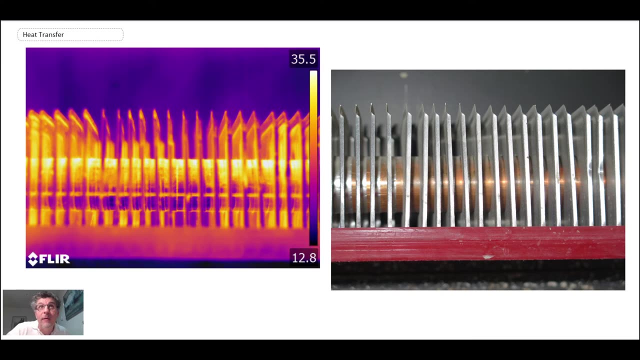 transfer. there's a refrigerator and you can see all the heat coming from the back on the ir camera and then, when you flip the refrigerator around, you can see the cooling coils. here is a radiator inside of the household and so it is heated. we have fins inside the radiator. hot fluid goes through the copper tube. 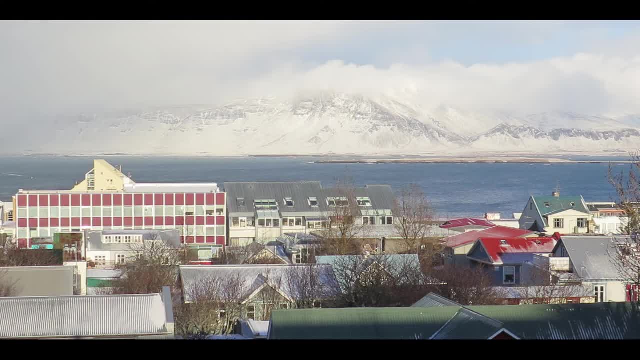 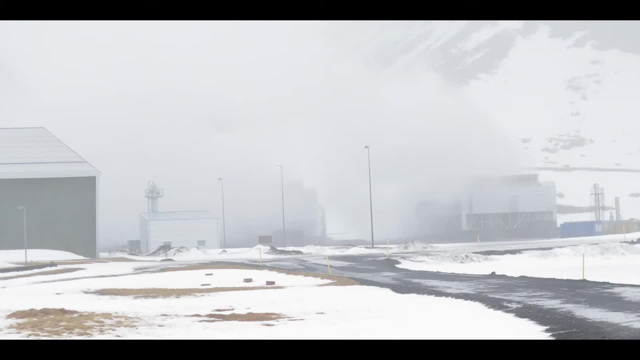 there are other applications. this is in reykjavik, iceland, and and they have very interesting for your natural convection with the geothermal power. they generate electricity from the steam, and so there you can see them generating the electricity in a turbine. they expand the steam. 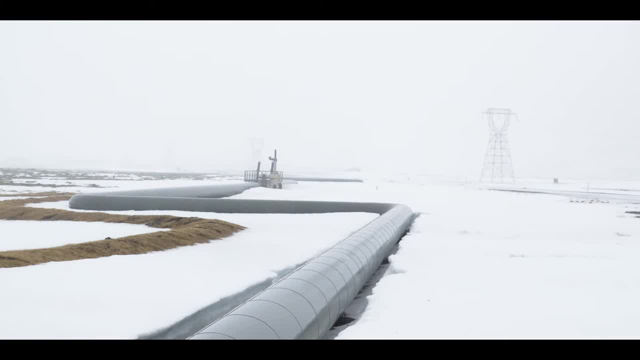 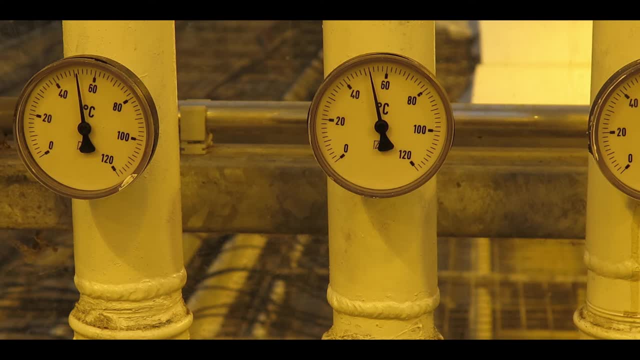 and the waste heat. they send that many, many kilometers to reykjavik and it is used for different applications along the way. here we have a greenhouse, and so the water comes in. it's about 52 degrees c. they then circulate it through these pipes on the bottom of the greenhouse.